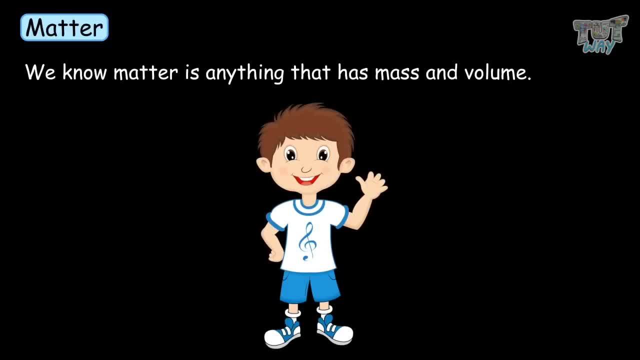 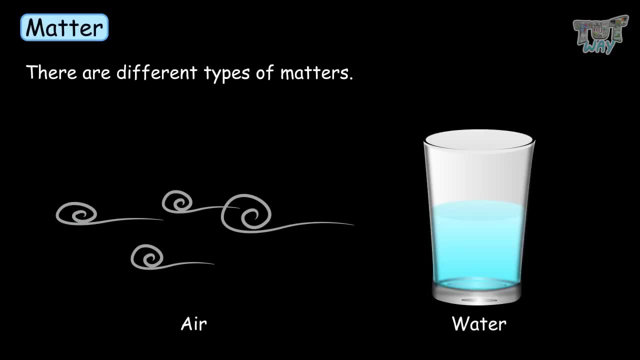 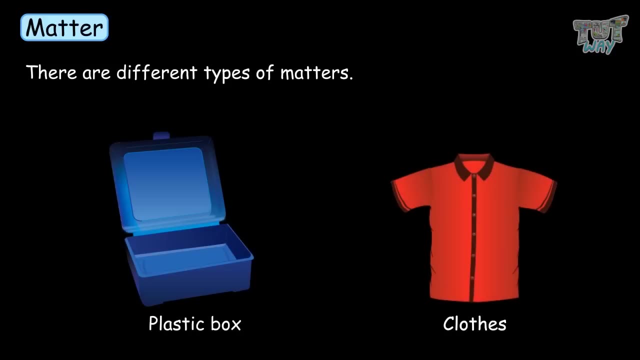 your bag, your home, you yourself are all made up of matter, But we see that there are different types of matter, Like air is different from water, Water is different from soil, Soil is different from your clothes. Your clothes are different from this plastic box. The plastic box is different. 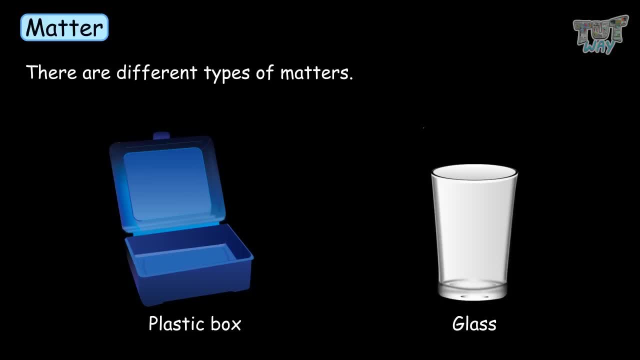 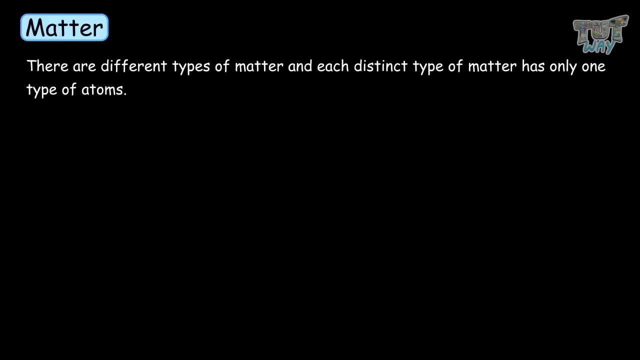 from this glass And so on and so forth. So there are different kinds of matter And distinct types of matter. only has one type of atom, So there are different kinds of matter And distinct types of matter are known as elements. For example, oxygen only has oxygen atoms. Nitrogen only has nitrogen. 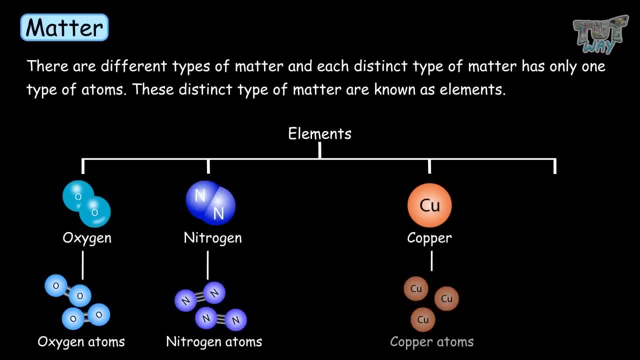 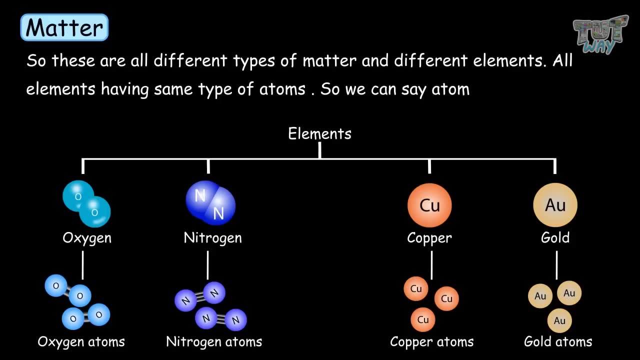 atoms. Copper only has copper atoms, Gold only has gold atoms. So these are all different types of matter and different elements, All elements that have the same types of atoms. So we can say the atom is the same type of matter, And so on and so forth. So there are different kinds of matter. 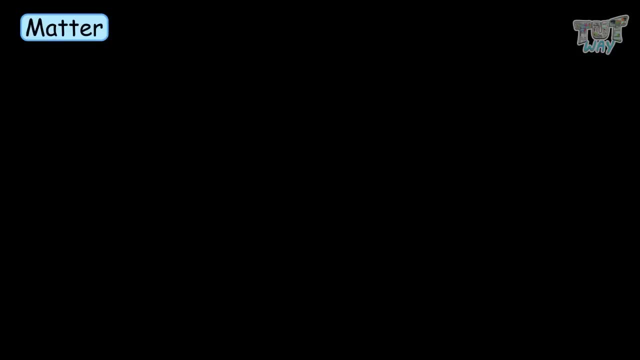 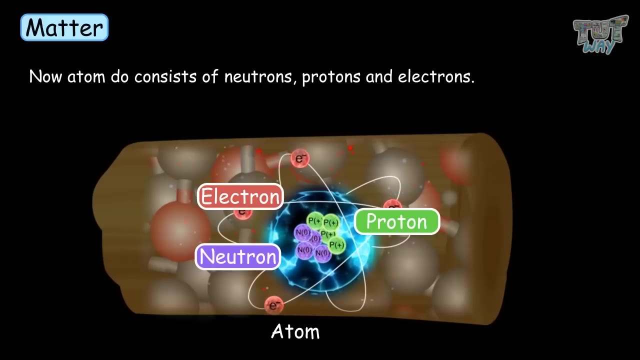 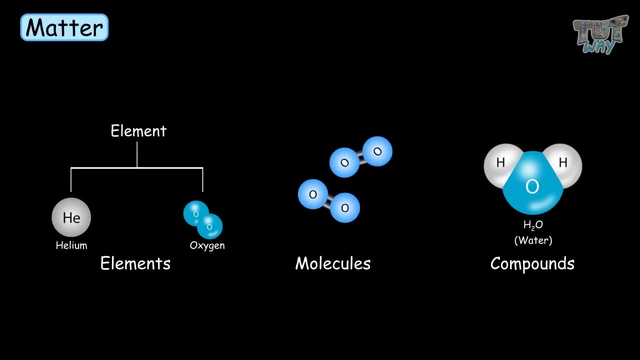 So there are different types of newsletter, There are different kinds of insurance, There are Watch A and D And these two longer various variables. Now, these two types of matter, they call the 21. Now we just want to first see what one of them represents. So what's this gas We can find? 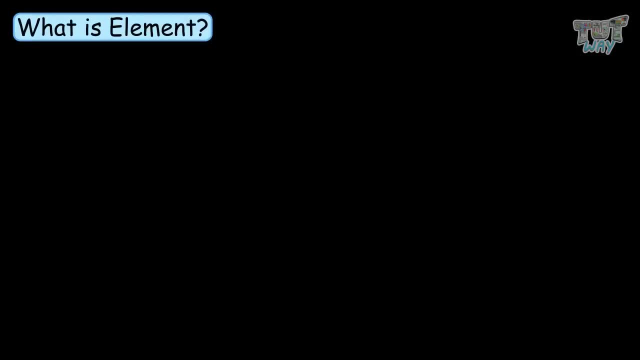 one of them. It's the small gas. It's supposed to be a little strong material. It's supposed to end at an altitude of 500 megabits. Isn't this the Lin li li Ins? This is an atom. So what this is? It's a. little guy. What isL está show? an element, Isn't it 것을? It's natural, but how does this create an element? Do they speak? No, it doesn't. So this is called an atom. This is the smallest unit of the. 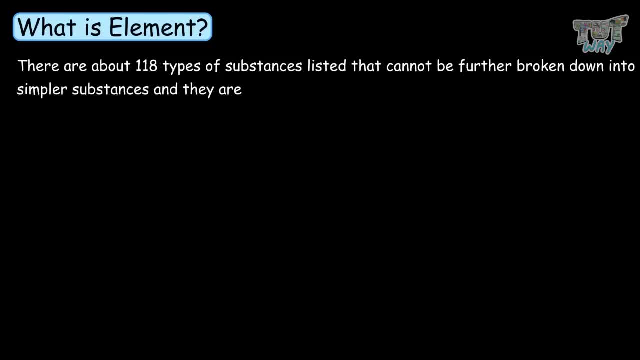 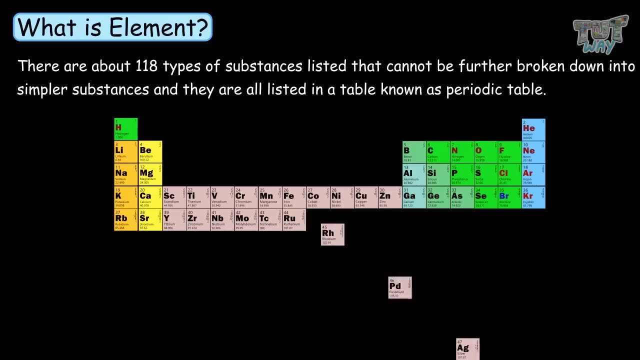 element, Now atoms, consists of a nucleus, protons and neutrons, But we will see the details, structure of the complacence into simpler substances, and they are all listed in a table known as a periodic table, as 118 types of different elements. This is the periodic table and all 118 types of elements. 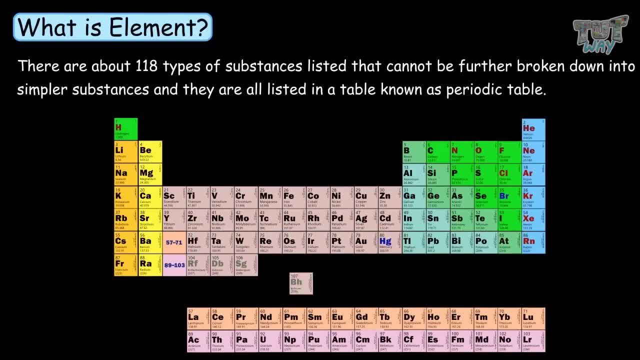 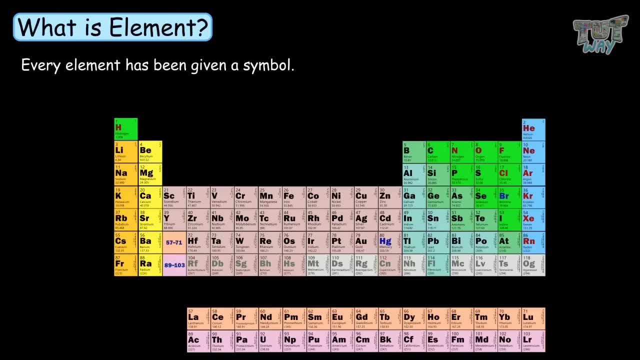 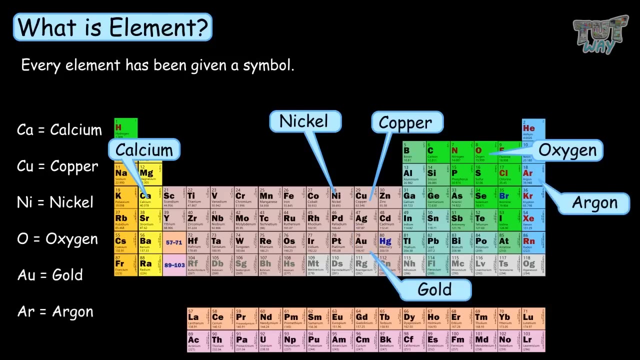 are distinct types of matter. They are listed in this table. Every element has been given a symbol: Ca stands for calcium, Cu stands for copper, Ni stands for nickel, O stands for oxygen, Au stands for gold, Ar stands for argon, and so on and so forth. And every element. 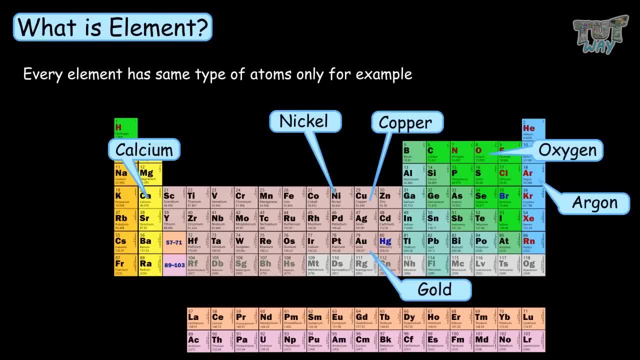 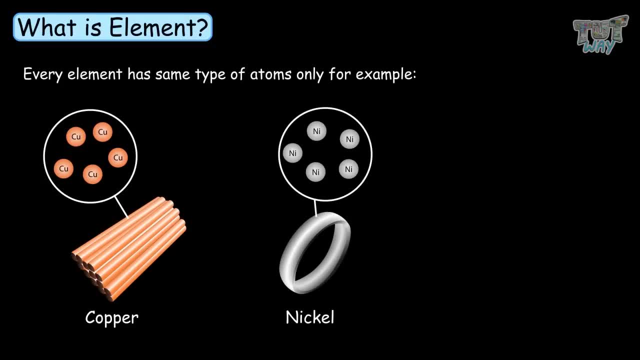 has the same type of atom only. For example, copper will only have copper atoms, nickel will only have nickel atoms, oxygen will only have teaspoon atoms, and so forth have oxygen atoms. So now we know what are elements. Now let's learn what are. 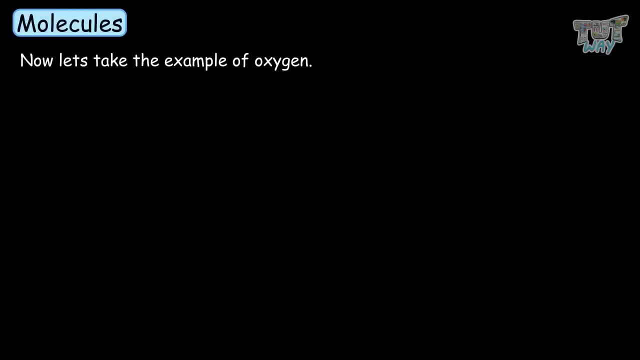 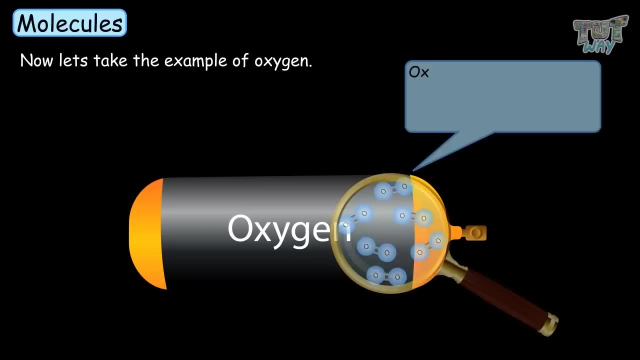 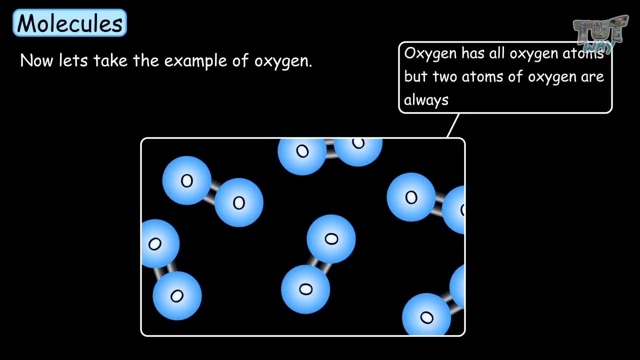 molecules. Let's take the example of oxygen. We learned that oxygen only has oxygen atoms. Now, in the case of oxygen, oxygen exists as a molecule that has two oxygen atoms bonded together. As in, oxygen is only oxygen atoms, but two atoms of oxygen are always bonded together, And this is why the formula of 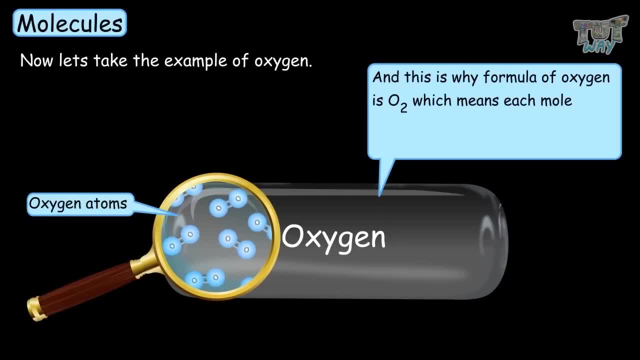 oxygen is O2, which means each molecule of oxygen has two atoms of oxygen in it And these molecules cannot be further broken down by ordinary chemical means. In this example of oxygen, we learned that oxygen has oxygen atoms and that oxygen is only one of two oxygen atoms. 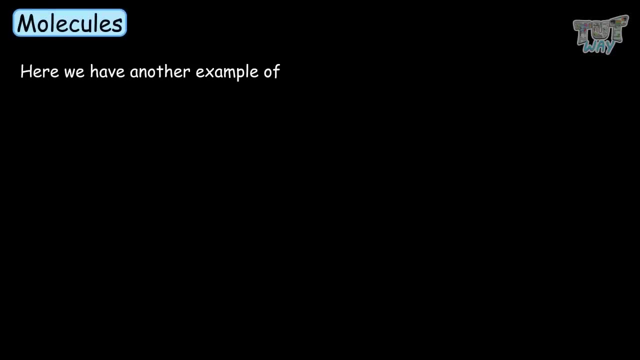 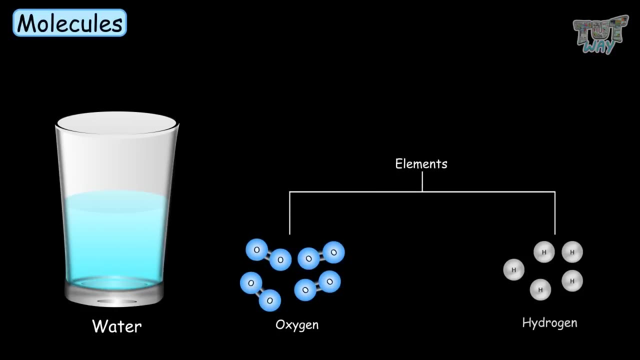 So now let's take the example of oxygen. We learned that oxygen exists as a molecule that has two. Here we have another example of molecules: water. Water is made up of two elements, oxygen and hydrogen, where water is molecules of water only, and each molecule is denoted as: 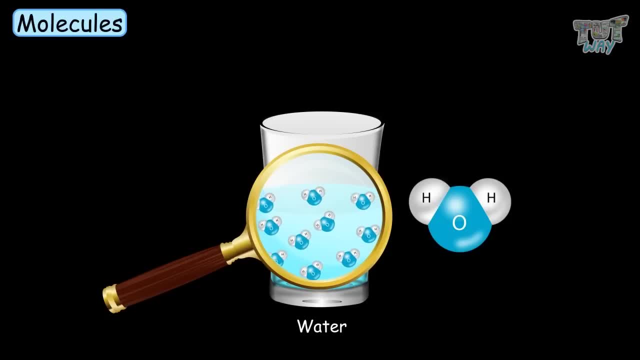 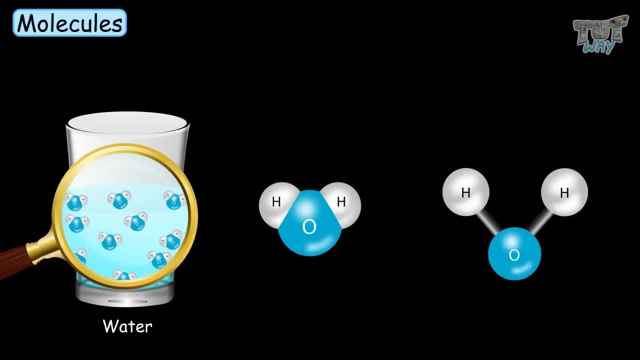 H2O, which means each water molecule has two atoms of hydrogen and one atom of oxygen. You cannot further break down this molecule into atoms by ordinary chemical means, so water exists as molecules of water. Each molecule has two types of atoms: hydrogen and oxygen. 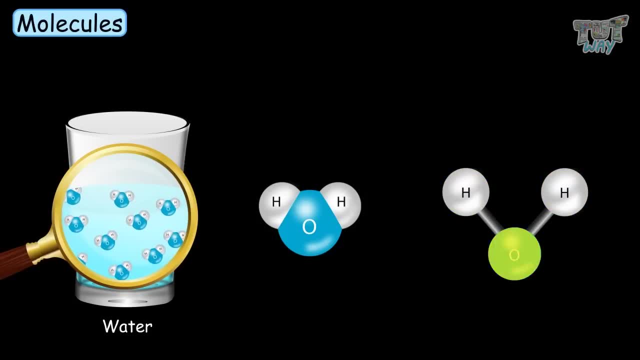 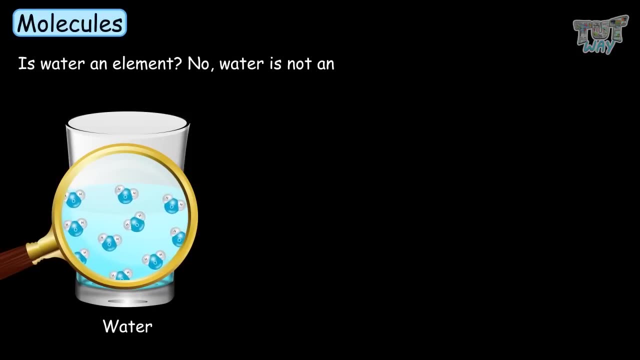 two types of hydrogen and one atom of oxygen. So is water an element? No, water is not an element. Water is a type of matter that has two types of elements- hydrogen and oxygen- and they exist as molecules. Each molecule has a composition: H2O. so let's revise it all again: Everything. 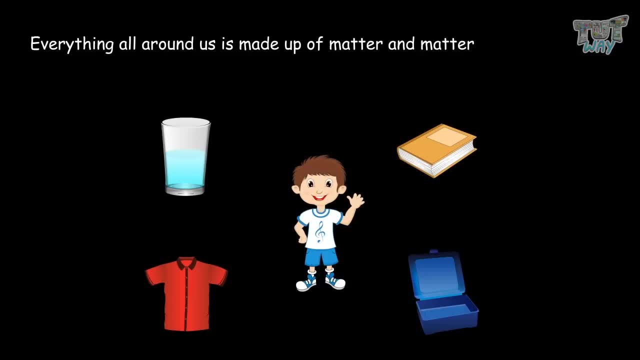 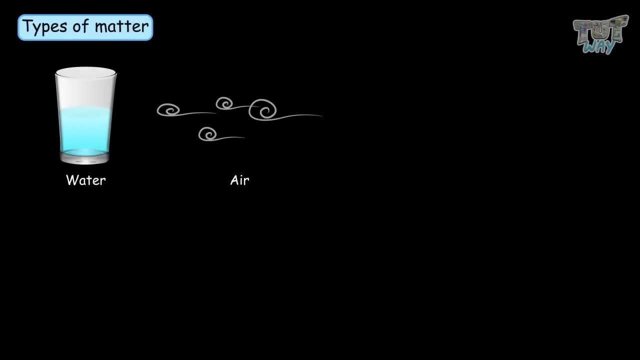 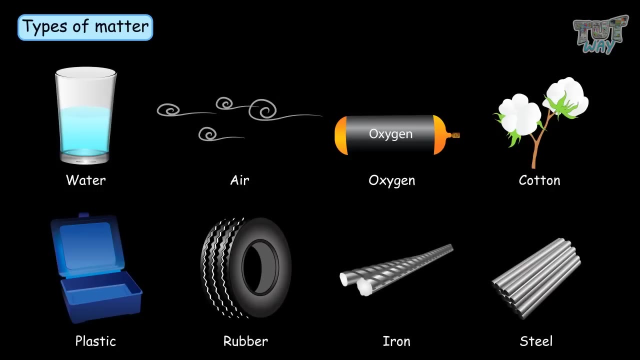 all around us is made up of matter, and matter is anything that occupies space and has mass, so water, air and oxygen. Water, air, oxygen, cotton, plastic, rubber, iron, steel- all of these are types of matter. 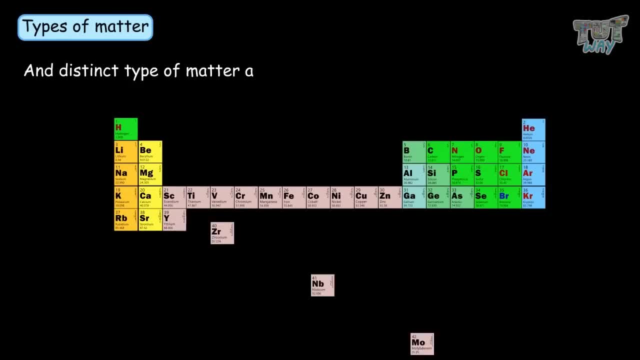 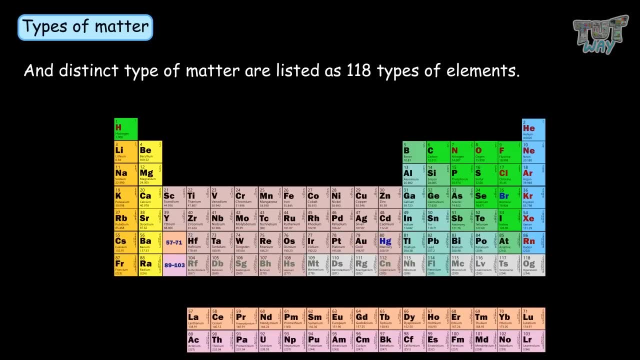 And distinct types of matter are listed as 118 types of elements, and they are listed in the periodic table and each element has a symbol. For example, hydrogen oxygen, nickel carmine and fl. Goldman's к hadn't hm. 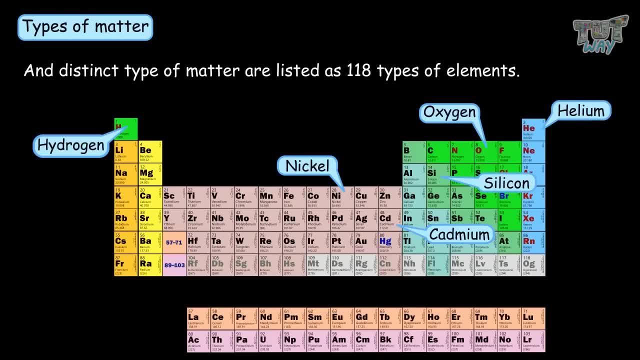 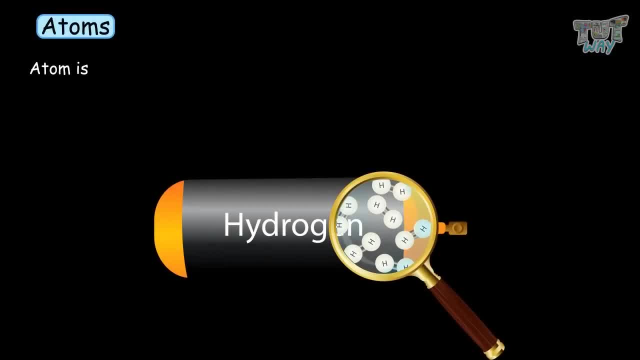 Cadmium, silicon, helium. All got distinct types of matter, As in, these elements have the same types of atoms. I did it already. So the atom is the smallest unit of matter. An atom exists as a molecule, as in they. 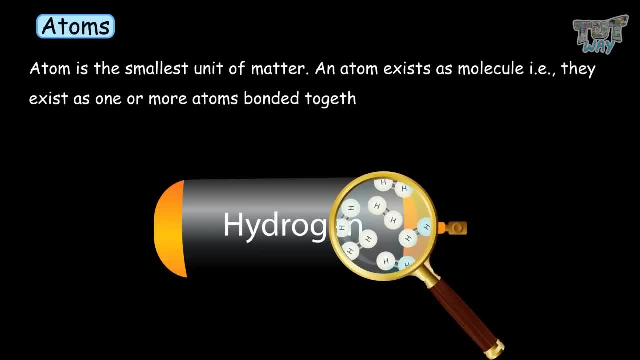 exist as one or more atoms bonded together, Like five muons being made up by aEE2O. These also exist as on beiden atoms. As an example –, воover, Pap Hiedrogen Oxygen exists as molecules of hydrogen, where each molecule of hydrogen has two atoms of. 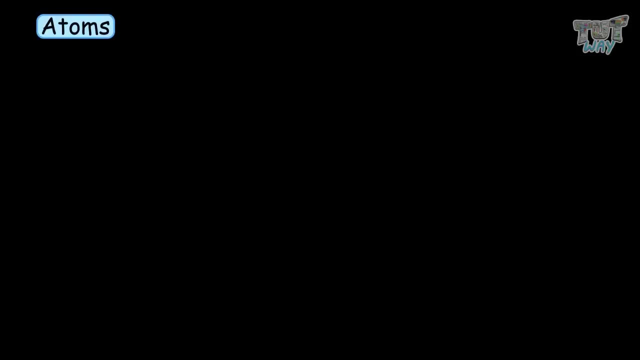 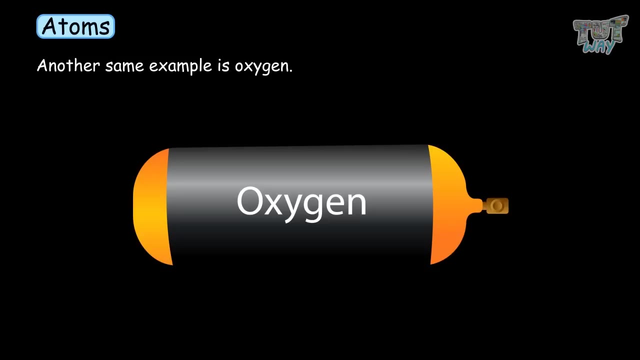 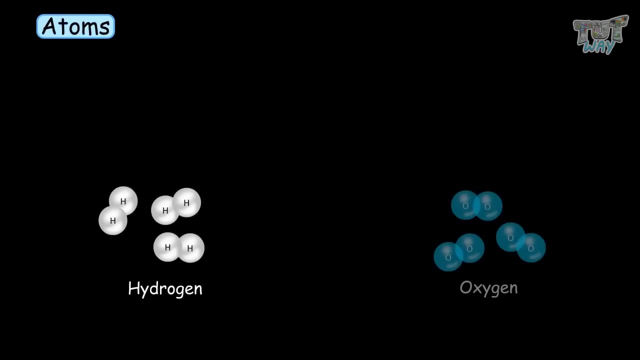 hydrogen bonded together. Another example is oxygen. Oxygen exists as molecules of oxygen, where each molecule of oxygen has two atoms of oxygen bonded together. So hydrogen and oxygen are elements because they have the same types of atoms, but some types of matter may not necessarily have the same atoms. 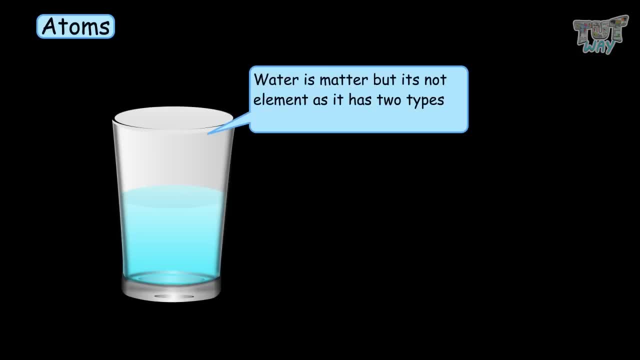 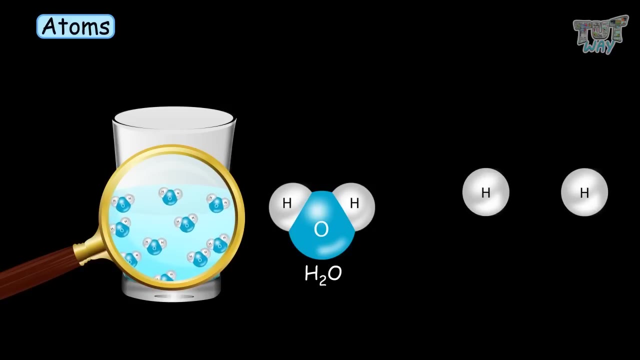 For example, water is matter, but it is not an element, as it has two types of atoms. Water has hydrogen as well as oxygen, and molecules of it exists as H2O. Two atoms of hydrogen and one atom of oxygen is there in each molecule of water. 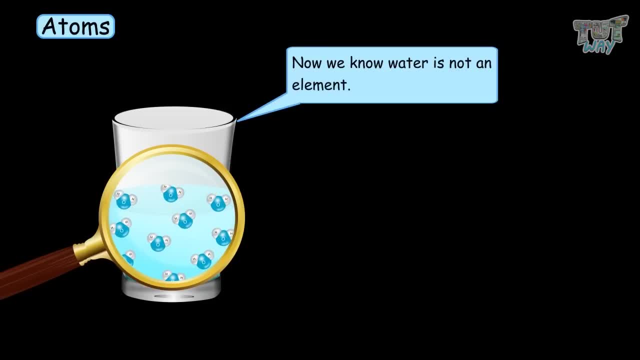 So now we know water is not an element. Then what is it? It is a compound, as in it exists of atoms of different elements in a fixed ratio. So we can say water is a compound of hydrogen and oxygen. Now let's have more examples of compounds. 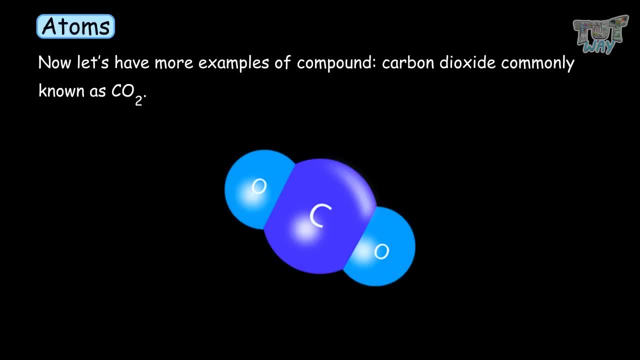 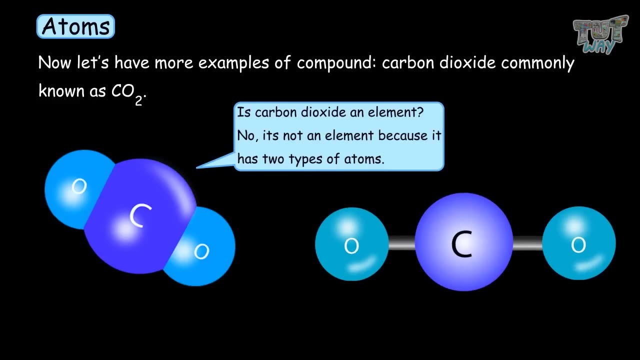 Carbon dioxide, commonly known as CO2.. So is carbon dioxide an element? No, it is not an element, because it has two types of atoms: Atoms of carbon and oxygen. So carbon dioxide is a compound, as in it is made up of two atoms of oxygen and one. 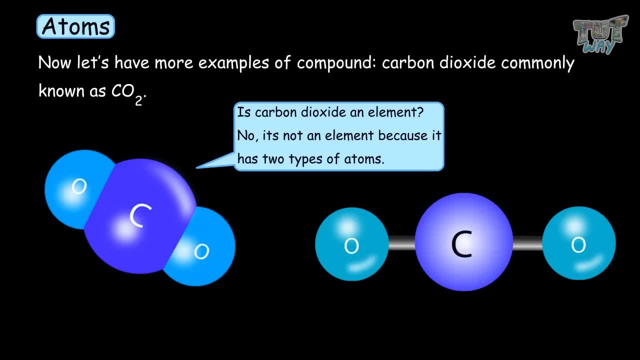 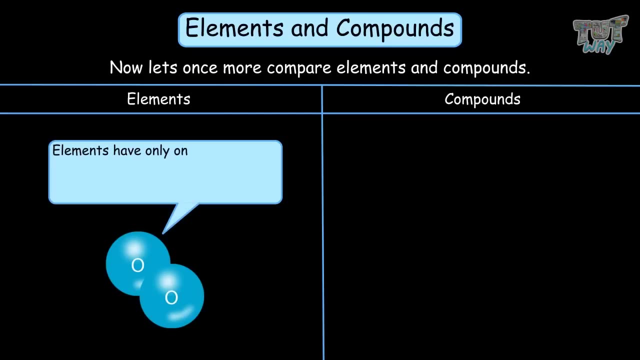 atom of carbon, as in all molecules of carbon dioxide have the chemical composition CO2.. One atom of carbon and two atoms of oxygen. Now let's compare elements and compounds. Elements only have one type of atom and each single atom has all the properties of. 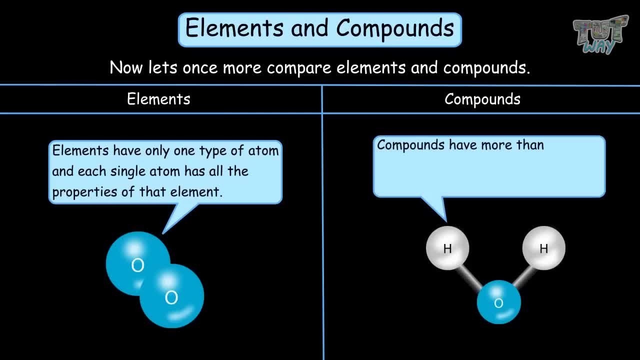 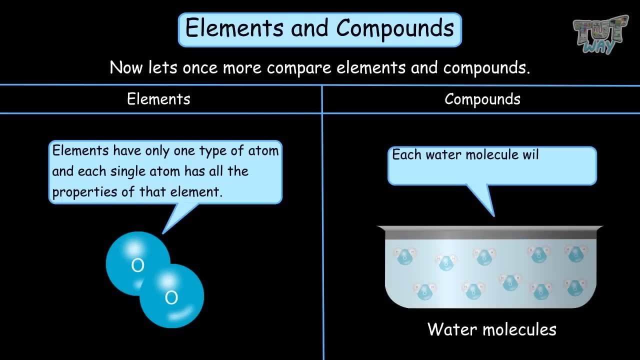 that element. Compounds have more than one type of atom bonded together in a fixed ratio in every molecule, and each molecule of a compound possesses all the properties of that compound, like water molecules. Each water molecule will have all the properties of water. Each molecule of carbon dioxide will have all the properties of water. 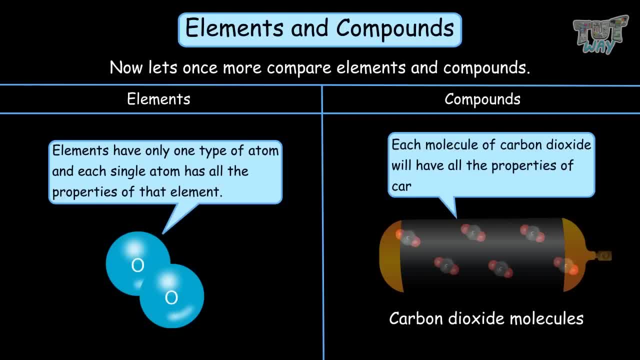 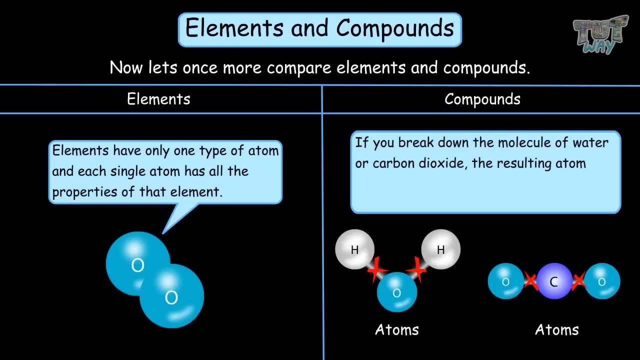 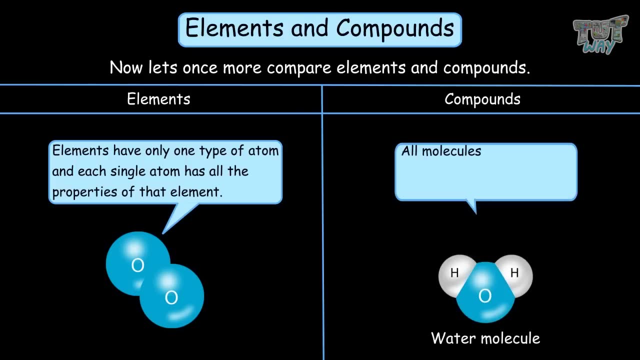 Each molecule of carbon dioxide will have all the properties of carbon dioxide. But if you break down the molecules of water or carbon dioxide, it will no longer have the properties of that compound. For example, all molecules of water have the chemical composition of H2O. 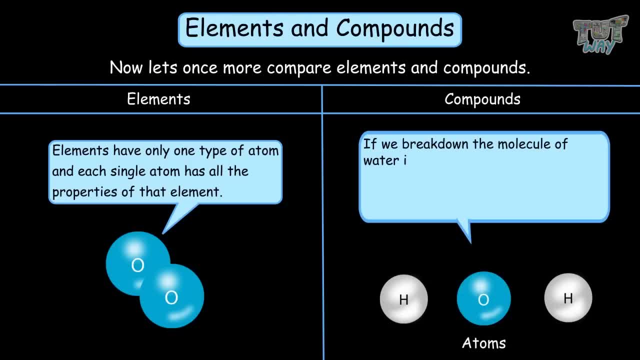 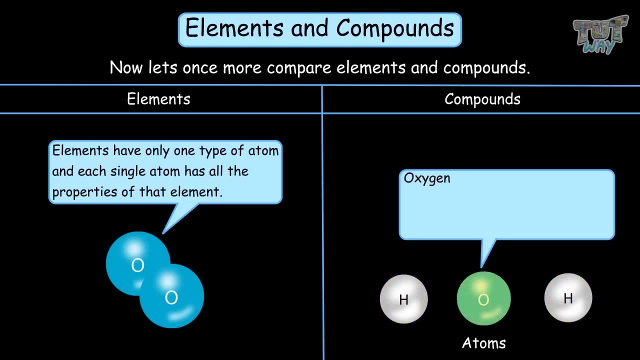 And if we break down the molecule of water as an H2O into its elements, as in if we separate hydrogen and oxygen, these elements will not have properties of water. Hydrogen will have the properties of hydrogen and oxygen will have the properties of the. 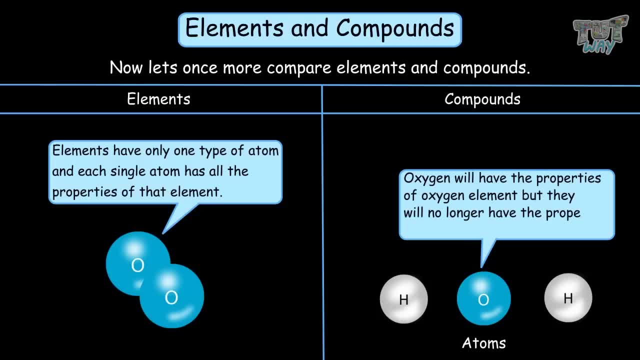 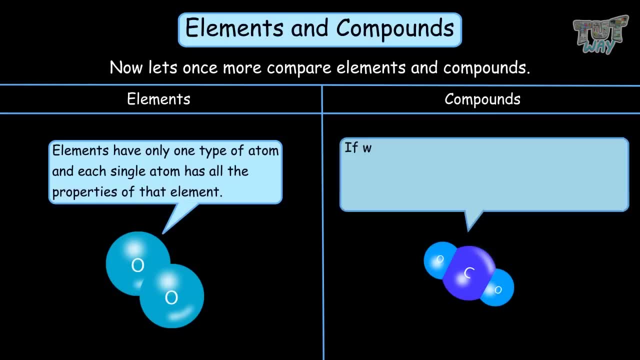 oxygen element, but they will no longer have the properties of the compound water. The same is true with the compound carbon dioxide. If we break down CO2 into carbon and oxygen, carbon will have the properties of the element carbon and oxygen will have the properties of the element oxygen. 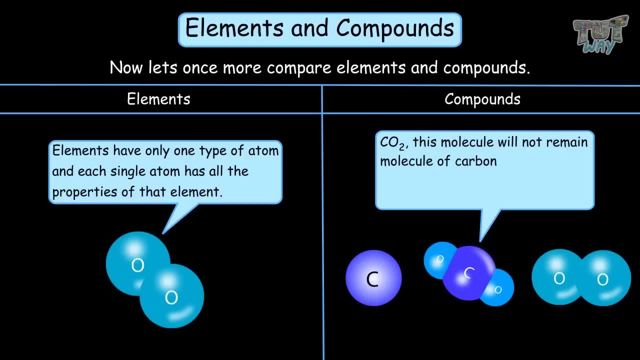 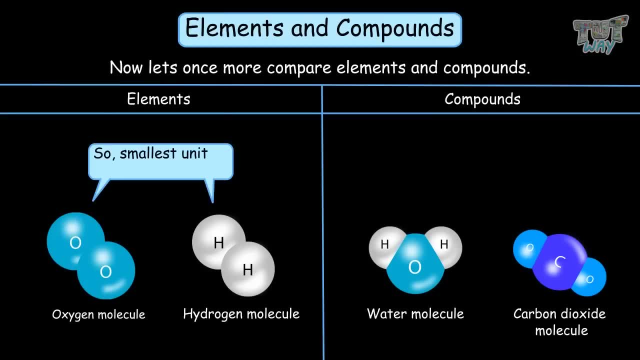 And this molecule will not remain a molecule of carbon dioxide and it will not have the properties of carbon dioxide. So the smallest unit of matter is the atom, and the molecule may have the same or different atoms and each molecule carries all the properties of that matter. 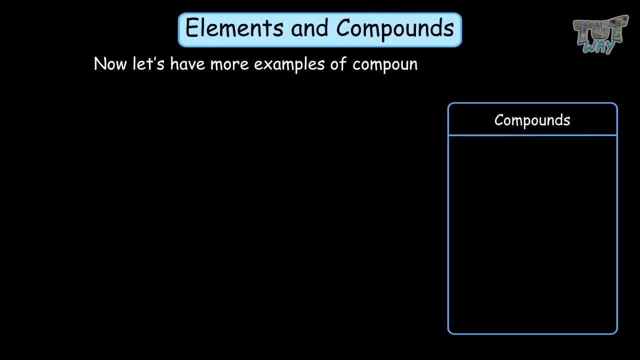 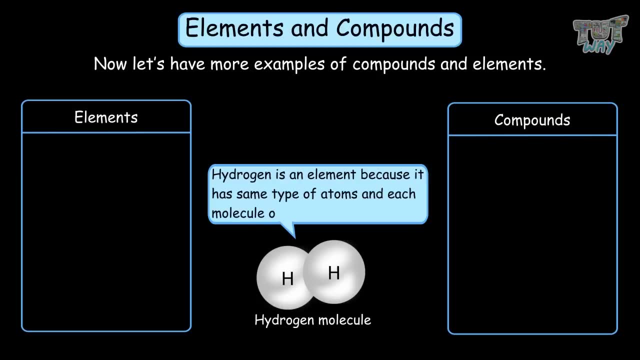 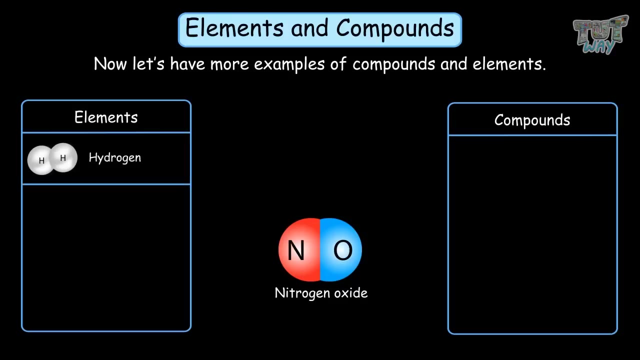 Now lets see more examples of compounds and elements. Hydrogen is an element because it has the same types of atoms and each molecule of hydrogen is H2.. Nitrogen oxide is a compound because each molecule of nitrogen oxide has the formula NO, as in one atom of nitrogen, and one atom of oxygen is there in every molecule of nitrogen. 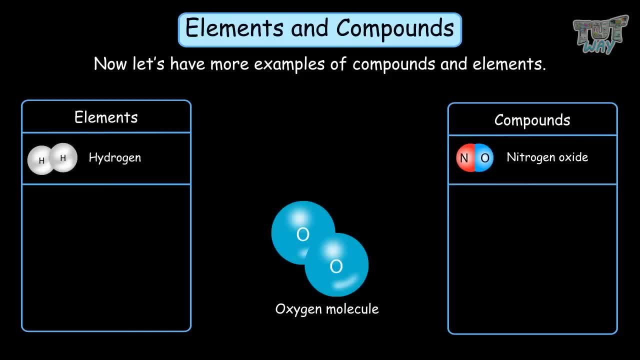 oxide. Oxygen is an element Because it has the same types of atoms. Oxygen And each molecule of oxygen has the same types of atoms and the formula is O2.. Nitrogen is also an element, Because the molecule of nitrogen has the same atoms. 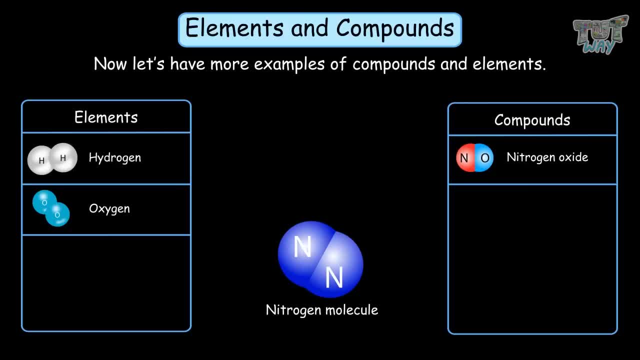 Only nitrogen atoms, And the formula is N2.. Chlorine: Chlorine is also an element, Not a compound, Because each molecule of chlorine only has chlorine atoms and the formula is Cl2. Water. So this is a compound. Each molecule of water has two types of atoms. 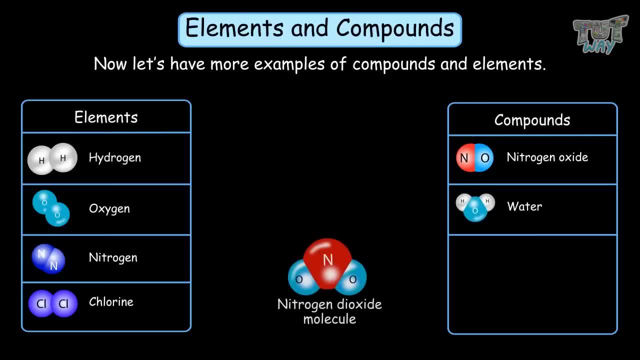 hydrogen and oxygen. Nitrogen dioxide: It is a compound, because each molecule of nitrogen dioxide has two types of atoms: nitrogen and oxygen, And the formula is NO2.. Carbon dioxide: It is also a compound, because each molecule of carbon dioxide has two types of atoms. 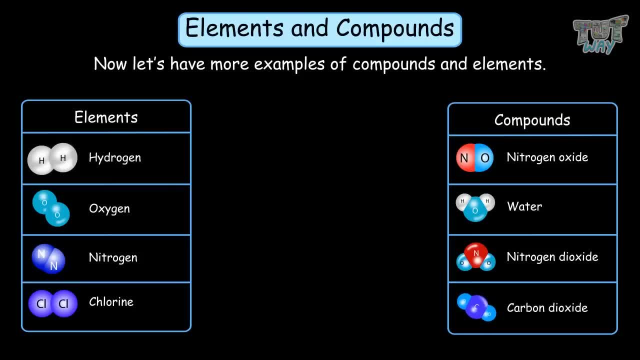 carbon and oxygen. So, friends, elements have the same types of atoms. Each molecule of an element has the same types of atoms, and the molecule is the smallest unit of matter that carries all the properties of that matter. Compounds have more than one type of atom.